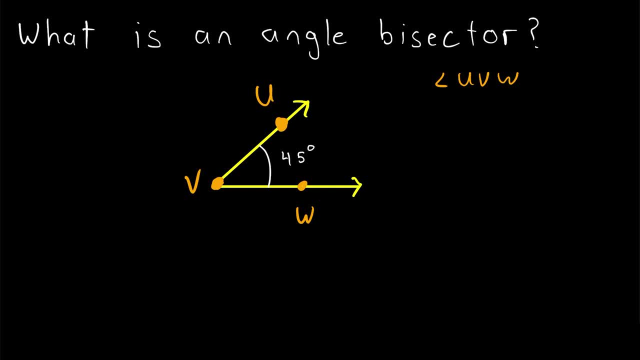 angle uvw where, remember, we always put the vertex of the angle in the middle. then an angle bisector of the angle uvw is just a line ray or line segment that cuts the angle into two congruent angles. So for this example, let's say we have this: 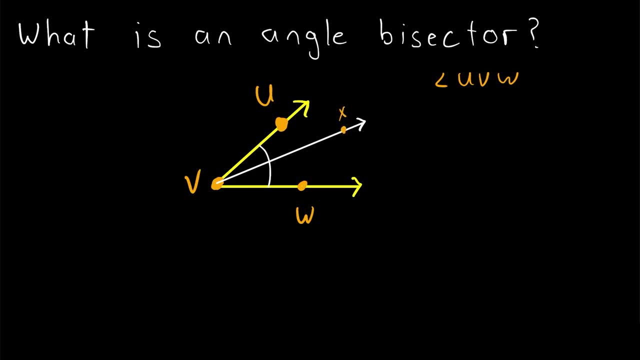 ray. We'll put another vertex on this ray, We'll call it x, And let me actually just redraw real quick so it looks more like an angle bisector. There we go. I think that looks about right. So if the ray vx is a vertex of the angle uvw, then the angle bisector of the angle uvw is a. 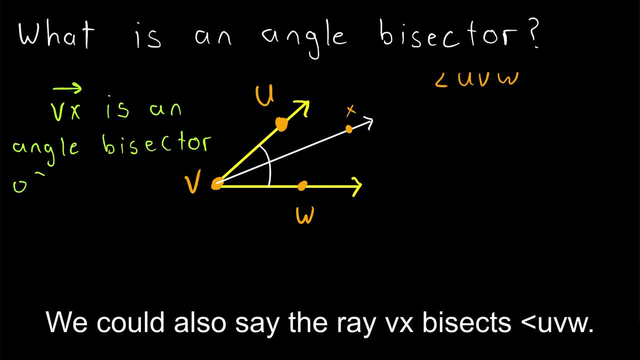 angle bisector of the angle uvw. That just means that the ray vx cuts the angle uvw into two smaller angles that are congruent. So we could draw some white hash marks to denote that these two smaller angles are congruent. So the ray vx sort of cuts uvw in half. So if the ray vx is an angle bisector, 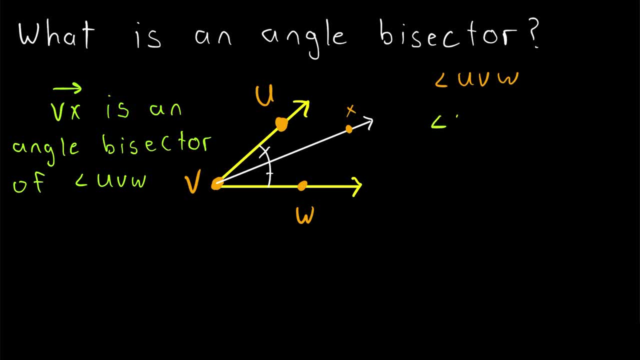 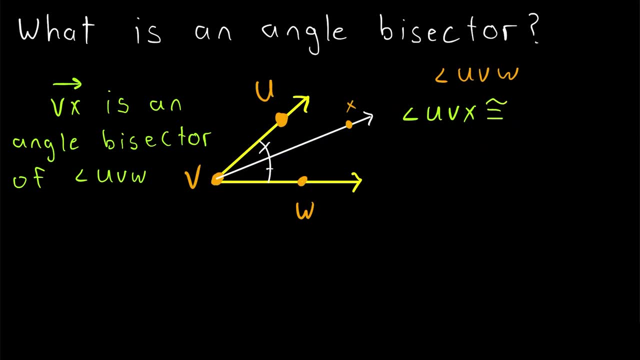 of uvw. then we could write that the angle uvx, that's this one here, is congruent. written like that is congruent to the angle xvw, this angle here We could also say that these two angles have the same measure, which we. 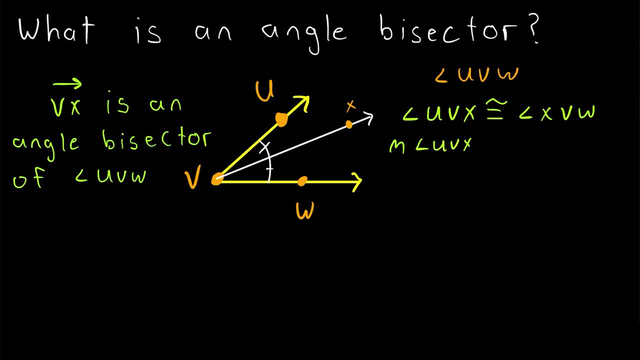 can write like this: m angle uvx. That means the measure of angle uvx is equal to m angle xvw, the measure of xvw. So if, for example, we have this angle uvw and vx is an angle bisector of uvw, and suppose we know. 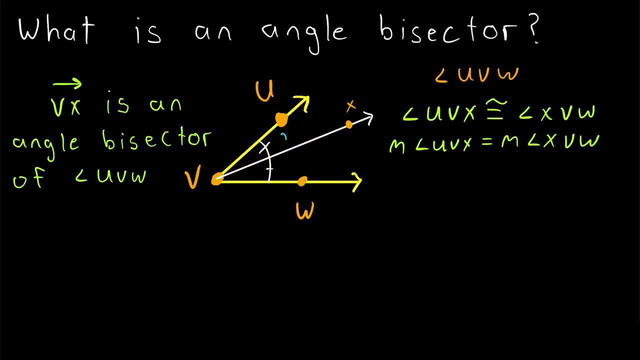 that angle. uvx has a measure of, let's say, 2x plus 3.. We could be picky and say that's 2x plus 3 degrees, but let's just leave the unit of degrees off, so it looks a little cleaner. 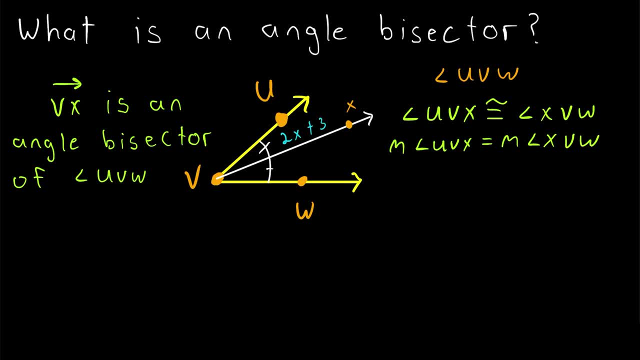 So suppose this angle uvx has a measure of 2x plus 3, and suppose that the angle xvw has a measure of, let's just say, 3x, Then how would we go about solving for x? It's very simple. 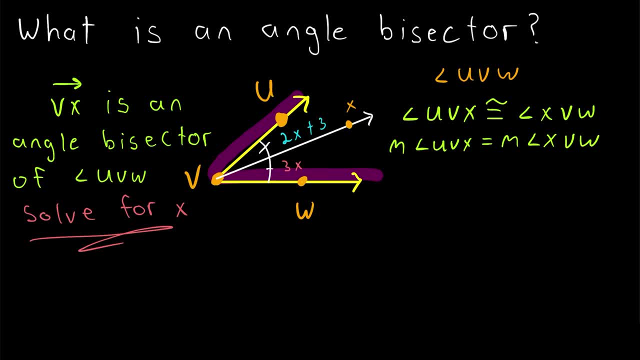 Since vx bisects the angle uvw, it must be the case that these two angles have the same measure. like we wrote over here, That's what it means for the ray vx to be an angle bisector. Thus we can solve for x by setting 2x plus 3 equal to 3x. These two angles have the same measure. 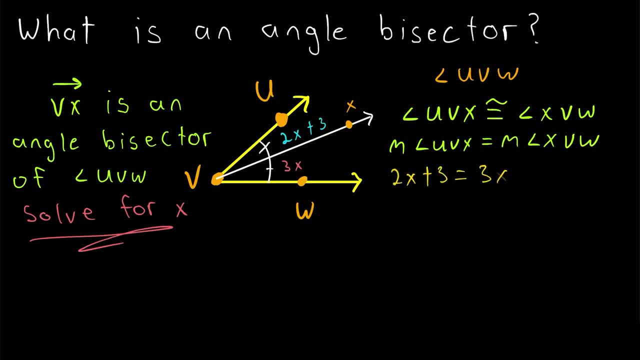 2x plus 3 is equal to 3x. Go ahead and subtract 2x from both sides and we'll be left with 3. on the left side of the equation is equal to 3x minus 2x, which is just a single x, And so that's. 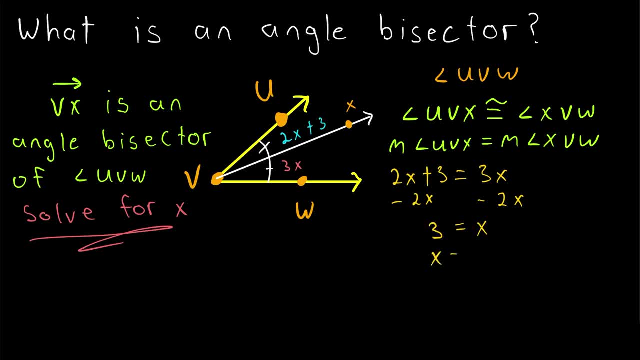 our answer: 3 is equal to x, or you might prefer to write, x is equal to 3.. And of course, this only works if we know that the ray vx bisects this angle. Otherwise, we have no way of knowing that. 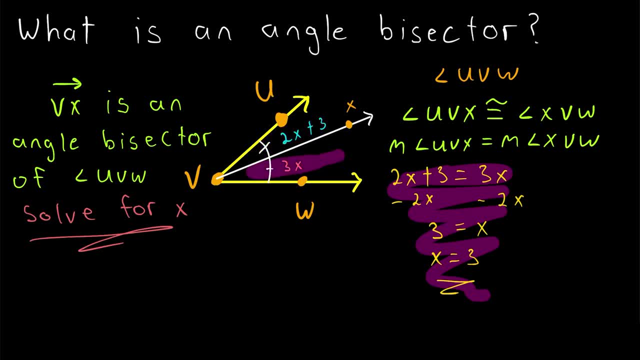 the measure of this angle- 2x plus 3, is equal to the measure of this angle 3x, And so that's what an angle bisector is. An angle bisector is a line, line, segment or ray that cuts an angle. 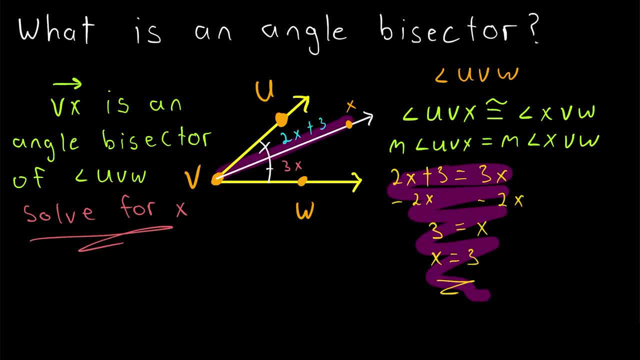 in half. It cuts the angle into two congruent smaller angles. So if these two smaller angles were not congruent- suppose uvx had a measure of 10 degrees and xvw had a measure of 13 degrees- then by definition vx would not be an angle bisector of uvw. So I hope this video helped. 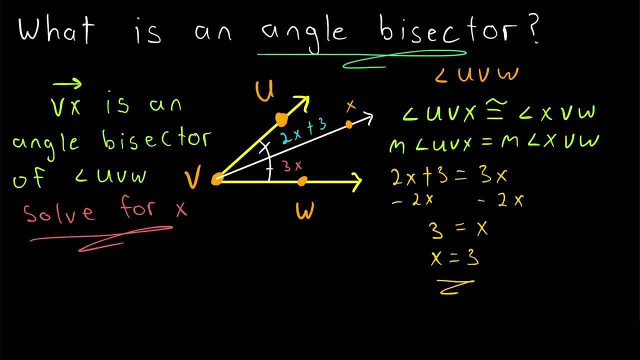 you understand what angle bisectors are and how we can use them to solve some fun little algebra problems. Let me know in the comments if you have any questions, need anything clarified or have any other video requests. Thank you very much for watching. I'll see you next time. 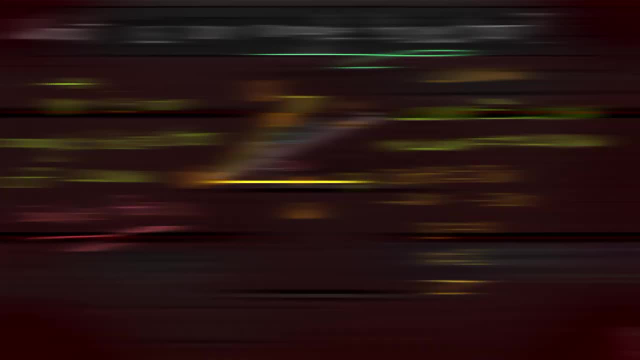 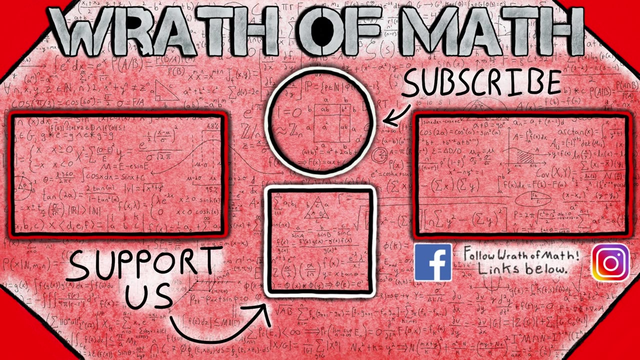 and be sure to subscribe for the swankiest math lessons on the internet. Thanks for watching.